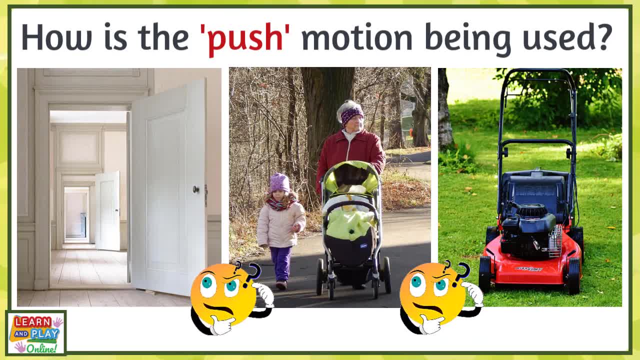 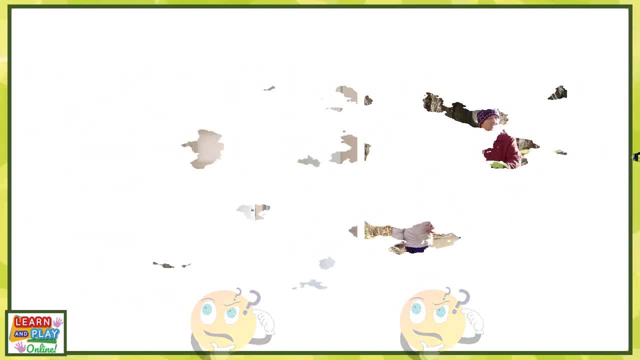 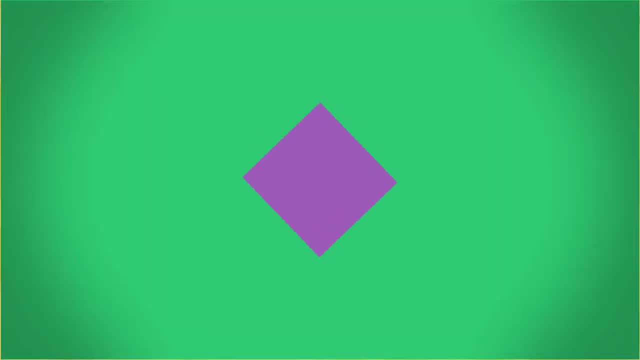 How is the push motion being used? Feel free to pause the video and discuss it with someone. Now that you are familiar with the force of pushing, let's move on to the other type of force that creates motion between objects, and that is the force of pull. 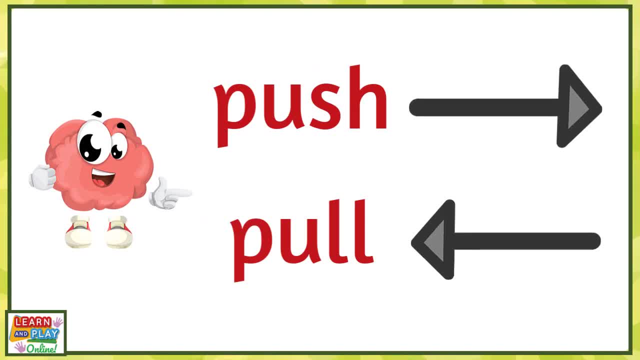 Did you know that push and pull are opposite forces? If they are opposite, then that means when you are pulling an object, you are bringing it closer towards you. Let's take a look at some examples of this. Have you ever flown a kite on a windy day? 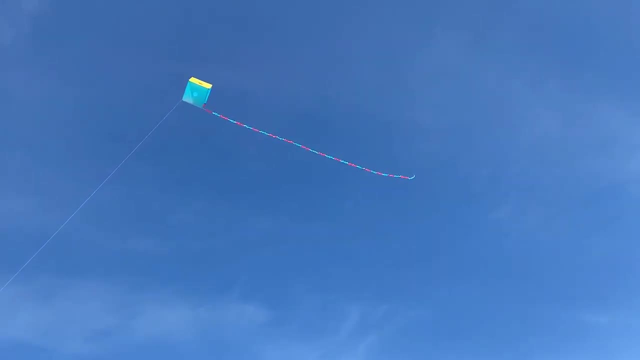 It is a lot of fun seeing your kite flying in the sky, but to make sure you don't lose your kite, you need to pull on the rope to keep it from flying away. Another example of a pulling motion may be motion is when fruit and vegetables are being harvested in order to pick the 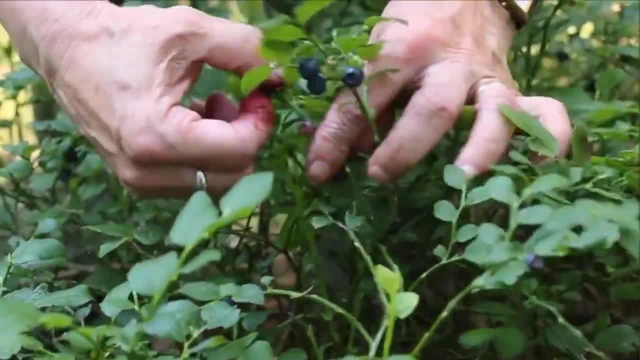 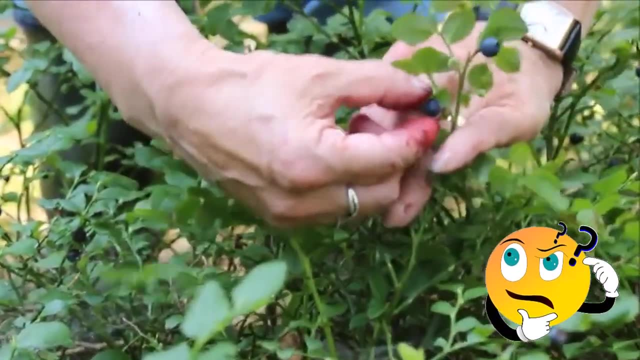 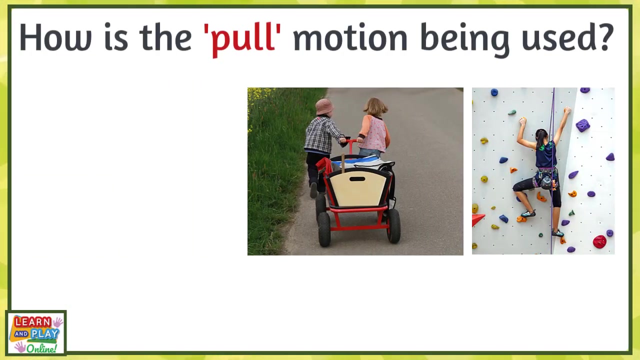 produce, you have to pull the fruit or vegetable away from the mother plant and bring it towards you. what other examples can you think of where the force of pulling is applied in real life? take a look at these pictures and try to answer the question. how is the pull motion being used? feel free to pause the video. 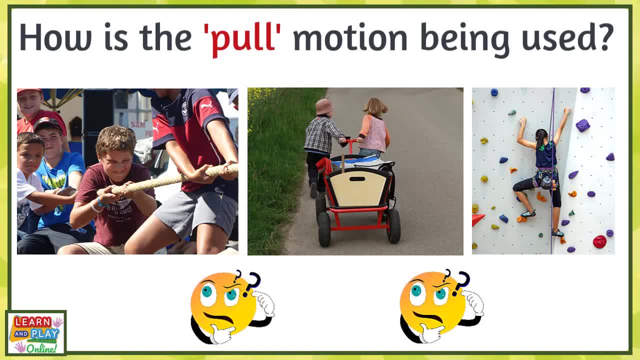 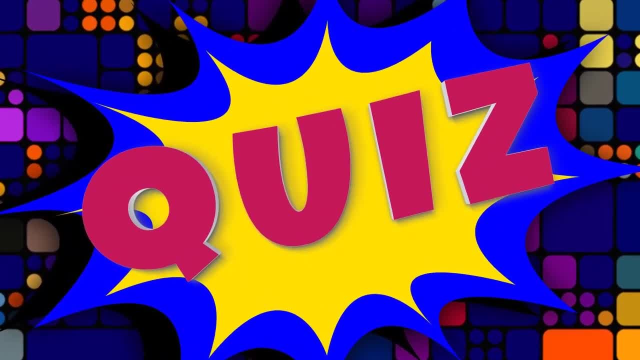 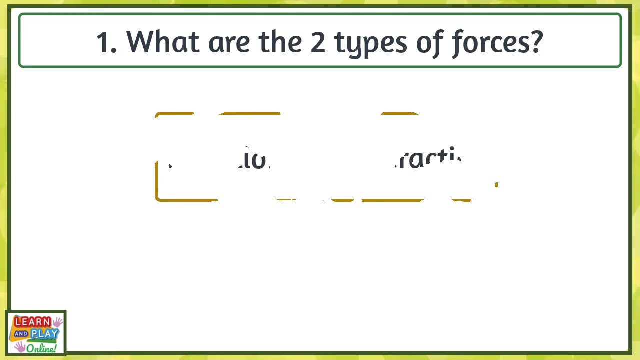 and discuss it with someone. now that you have learned about the push and pull forces, it's time for a fun quiz. question 1: what are the two types of forces: motion and interaction or push and pull? question 2: how can you define a push, a motion that moves objects away from you?